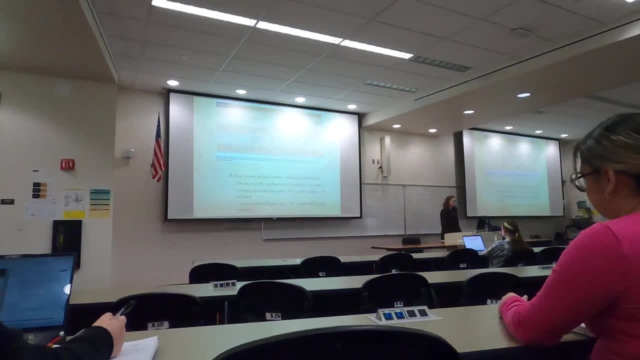 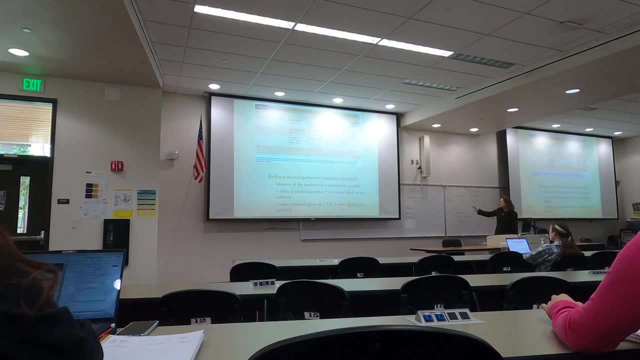 And this is what's on this slide here. I put this up on here because it's handy to just like look back at this as we're looking at each thing that these microbes are doing. Okay, so these are the three ways that microbes can make nitrogen available. So this is available to be part of the amelioration process. 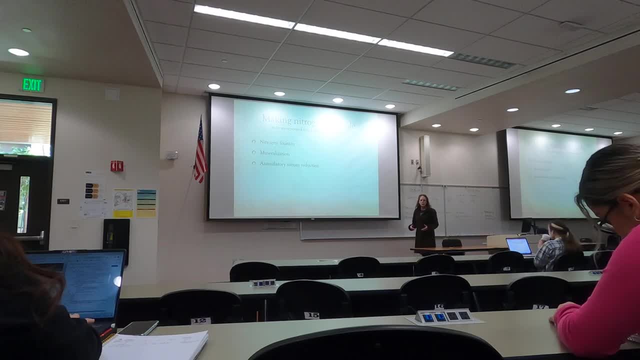 So this is the amino group and the amino acids that are going to be part of the proteins, Or be the nitrogen that's part of the nitrogenous bases, the adenine, guanine, cytosine, et cetera, that would be part of the nucleotides that then will be part of DNA and RNA. And so let's take a look at all three of those things. First, we'll start with nitrogen fixation, And this is what we're going to do. So this is what we're going to do. So this is going to be a reduction. So it's going to take N2 and convert it to ammonium. 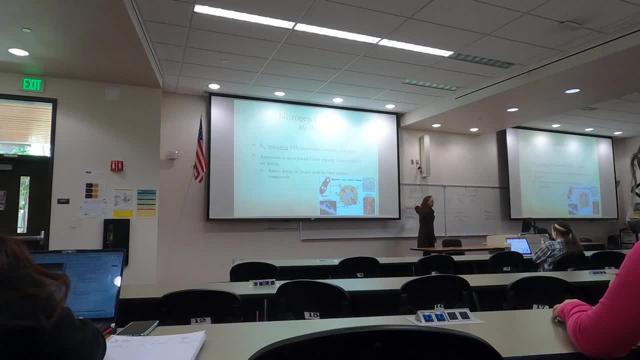 And then this can be used in the amino groups of the amino acids and so forth, to be incorporated into proteins and also the DNA and the RNA. Obviously not with the amino acids, though, These nitrogen fixing organisms- here's an example of one. There are many. 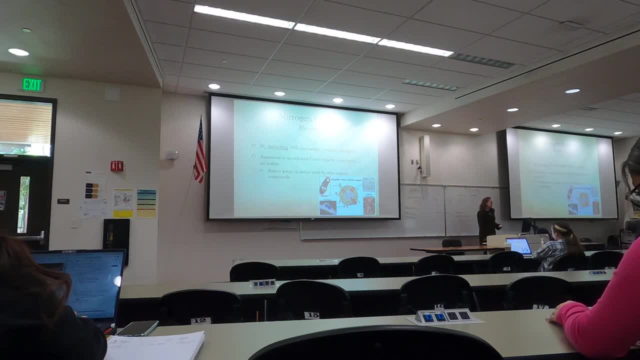 Rhizobium is an example of one. We learned about that for our last exam that we had. This organism infects the root nodules of legumes- These are things like clover, peas, alfalfa- And it has a symbiotic relationship with those plants. But there are also nitrogen. There are nitrogen fixing bacteria that are free living, that aren't associated with the root nodules of plants. But what is interesting, if you're like into agriculture, like growing crops and things, having growing legumes on that cropland at various points in time can add to the nitrogen- the available nitrogen for other plants in the future because of this symbiotic relationship. 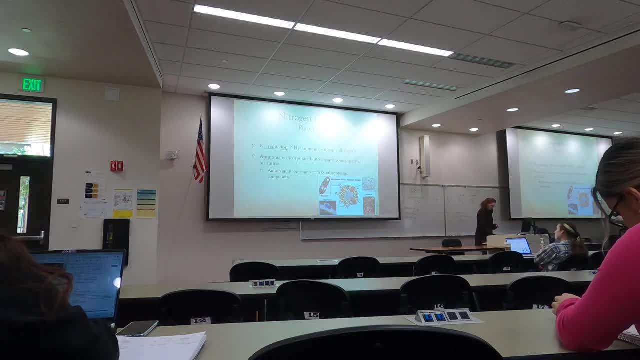 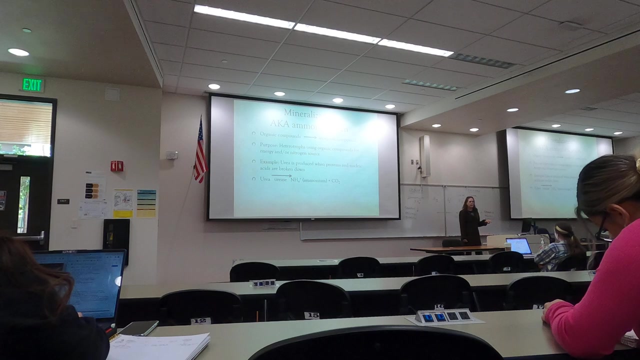 So this is going to take N2 into the air. You convert it into a form that can be incorporated into proteins and nucleic acids. This is another way of making nitrogen available, but not taking N2 and doing something with it. This is the part where microbes are breaking down organic compounds like the dead plant and animal matter. 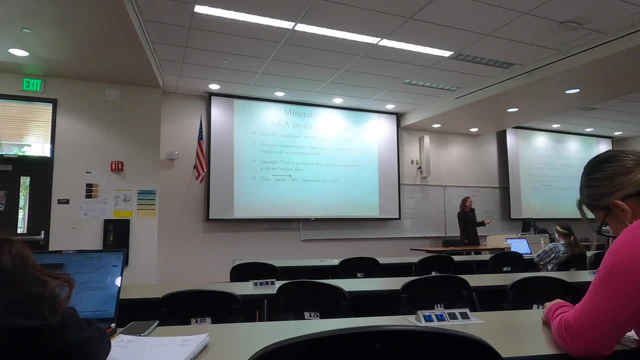 So they're breaking down the proteins and the DNA and organic compounds. So they're breaking down the proteins and the DNA and organic compounds. So they're breaking down the proteins and the DNA and organic compounds. So these would be heterotrophs that are using those organic compounds for energy and or also a source of nitrogen for them.